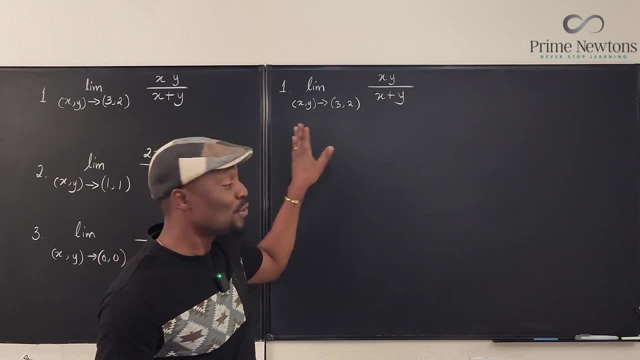 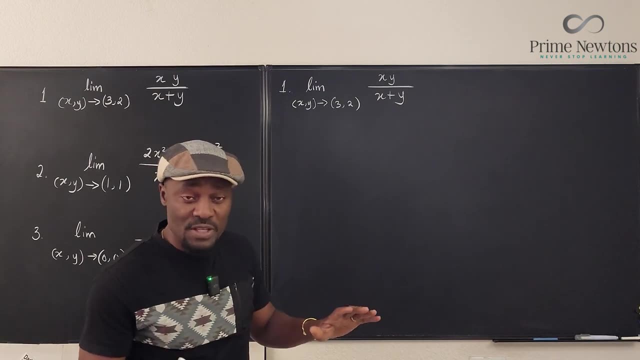 point and see what you get. And that's what you do every time you get a limit problem, Because the numbers here are 3 and 2, there's no infinity. What we do first is we try to plug in the numbers If it works out. 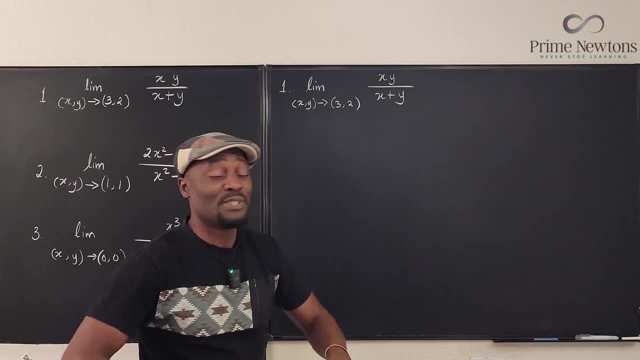 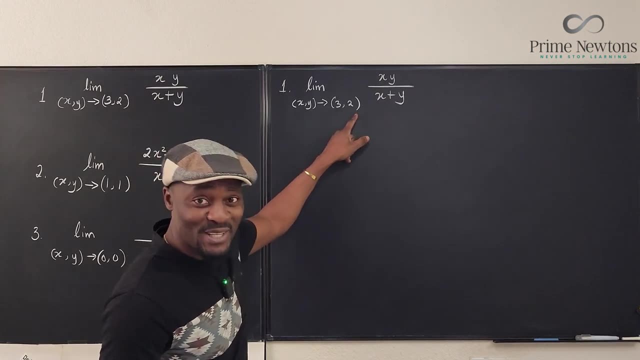 then that's our answer. If it doesn't work out, then we have to devise a strategy. So let's plug in 2 for x and plug in 3.. I mean, plug in 3 for x and plug in 2 for y. This is going to be equal to: 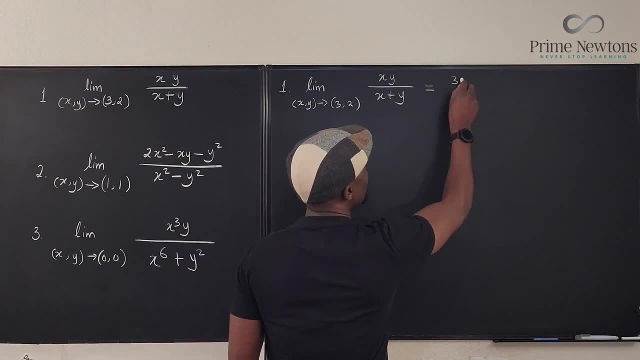 if I plug in 2 here, it's going to, I mean, 3 is going to be 3 multiplied by 2, divided by this is going to be 3 plus 2, and my answer is 6 over 5.. I'm done, That's the limit. 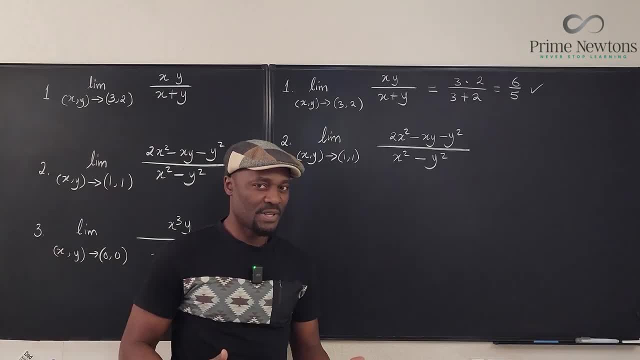 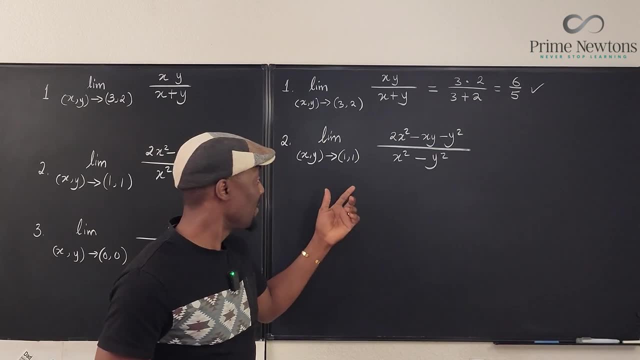 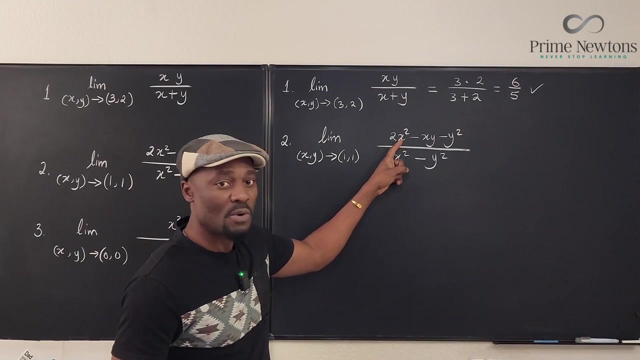 It's easy, right? Okay, let's go to the next one, This one. it's another finite point that you're given, So the first thing you do also is to plug in the numbers. So if I plug in 1 for x and plug in 1 for y, this is what's going to happen. This is going to become 2 times 1. 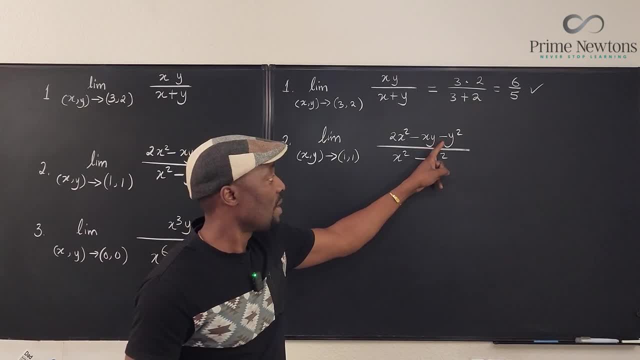 minus 1 times 2.. This is going to become 2 times 1 minus 1 times 2.. This is going to become 2 times 1, which is 1 minus 1 times 1, which is 1.. So it's 2 minus 1 minus 1, which gives me 0 on top In the 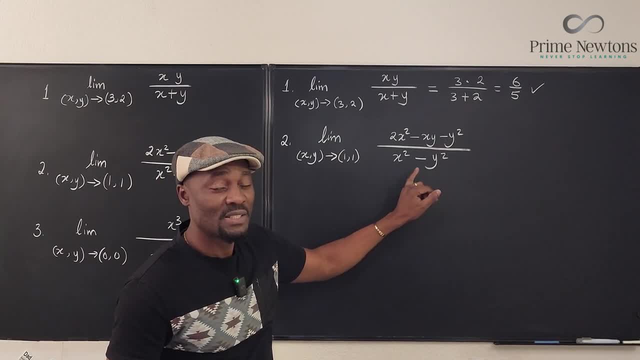 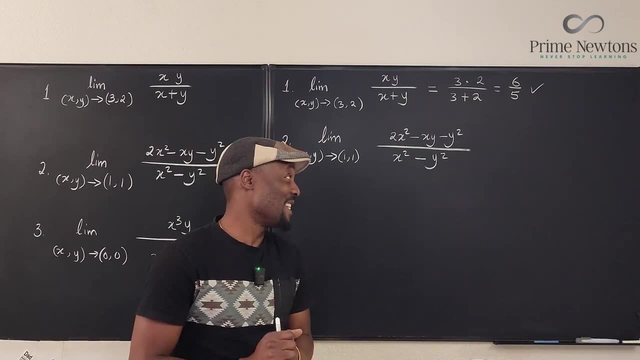 bottom, I'm going to get 1 times 1 minus 1 times 1, which is 0. So I have a 0 over 0, 0 situation. The problem in this case is we're not going to be using L'Hopital's rule, So you better know how to. 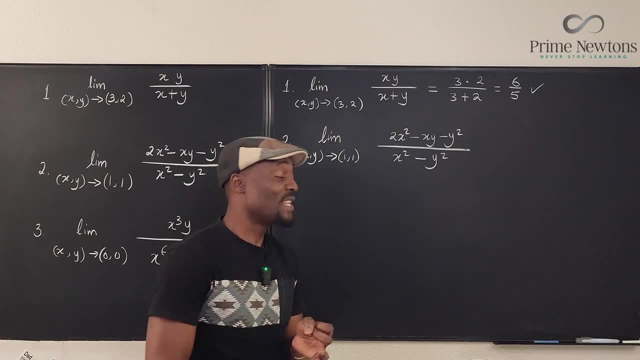 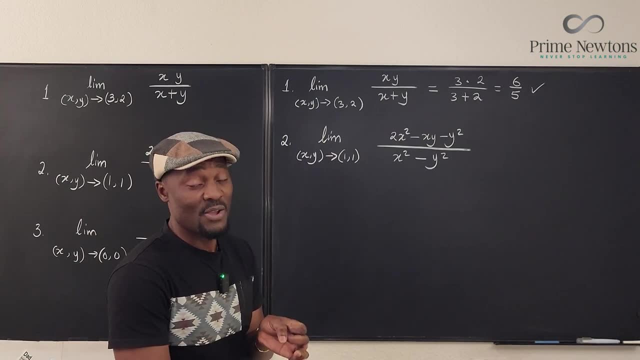 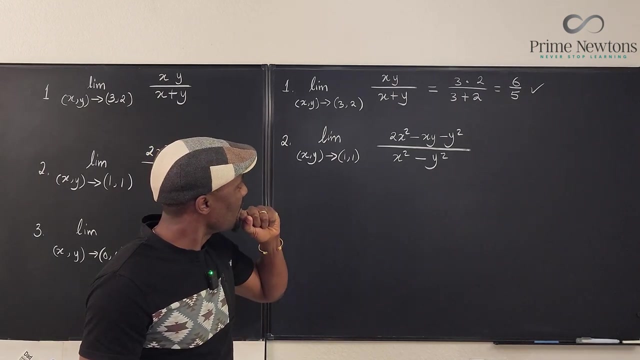 do your factoring or use other strategies that are used in this case. So if I cannot use L'Hopital's rule, factoring must be my greatest strength when it comes to this kind of exercise. So how can we factor, just to see what can come out of this? Can we factor this? Is this a quadratic? Yes, 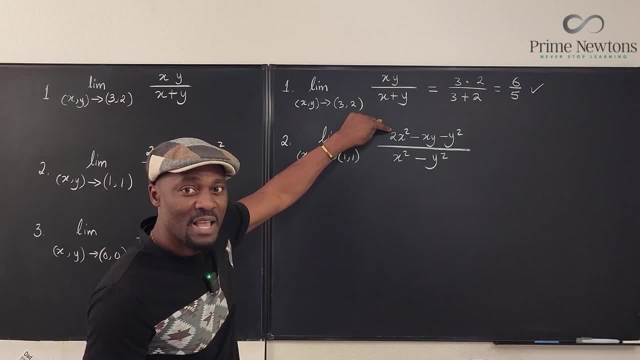 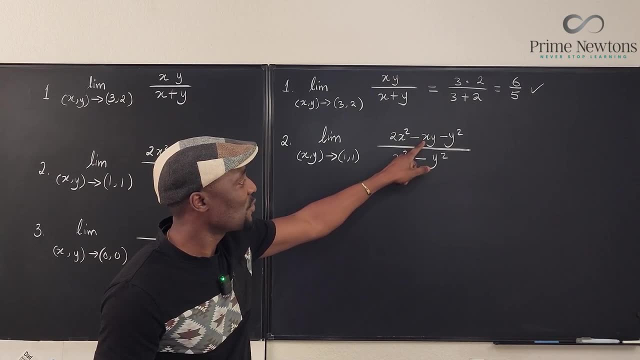 actually this is a quadratic, because you can factor this by splitting this in the middle and writing it instead as minus 2xy plus xy. Okay, you have to be able to do that. So what I'm going to do is say: this is my greatest strength when it comes to this kind of exercise. So I'm going to 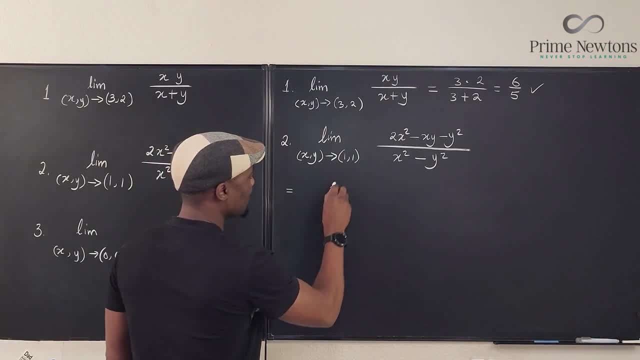 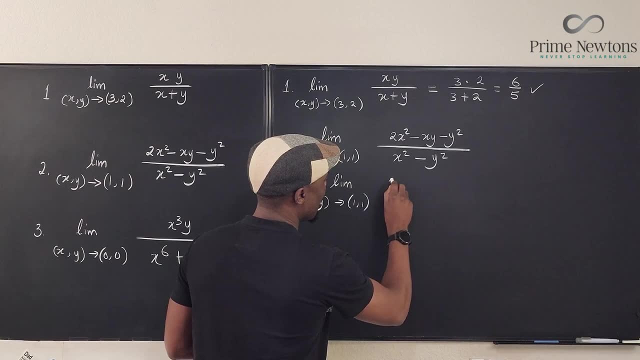 this is equal to the limit as the point xy approaches the point 1, 1.. We have 2x squared minus 2xy, plus xy, minus y squared. Okay, divided by x squared minus y squared. Now, how did I know? 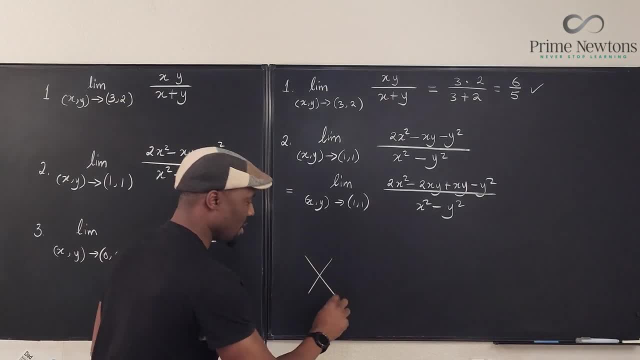 this is what I'm supposed to write. Well, I just solved that. Remember that puzzle thing. You multiply 2 by minus 1, you get minus 2.. So I'm going to do that, So I'm going to do that, So I'm. 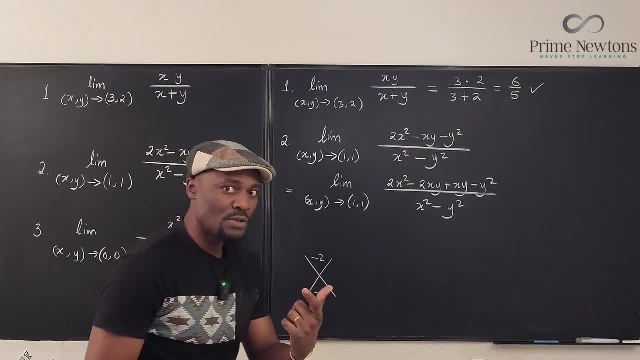 going to add 2 to x, squared minus 2, and then the bottom is minus 1 and you say: what two numbers will I multiply to get minus 2? and if I add them together I'm going to get minus 1. while it's. 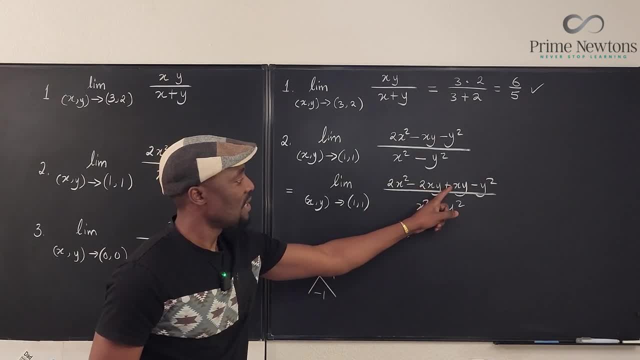 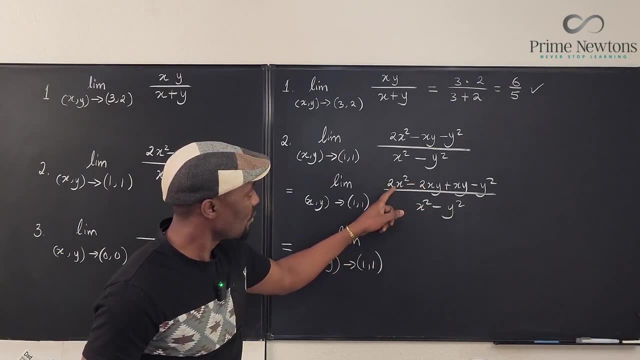 minus 2 times 1, and that's what I just did, minus 2 times 1.. So if I factor this, what I'm going to get would be what's common to both of them. I can take out 2x, So I'm going to end up with 2x. 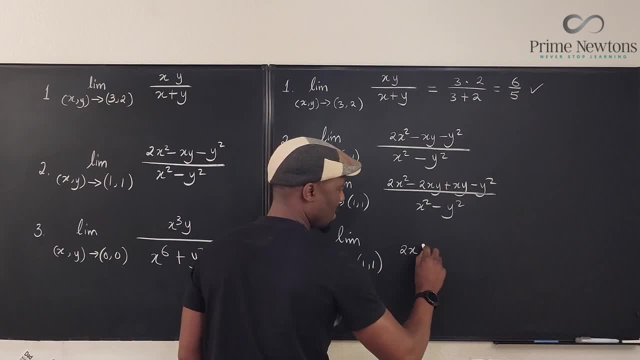 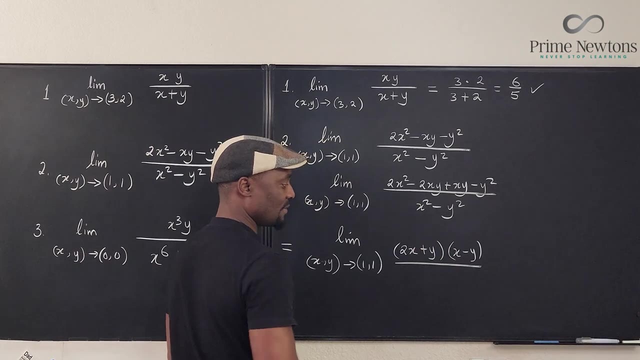 What's common to these two? it's y 2x plus y. Okay, and what's going to be left on the inside is going to be x minus y, x minus y. over now, this is difference of two squares. i can write it as x plus y times x minus y. okay, so clearly this can cancel this out. so you see that. 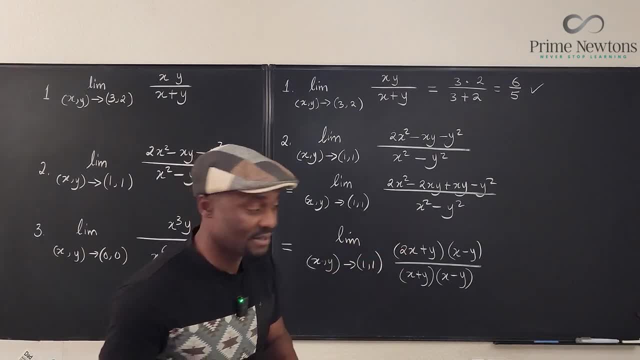 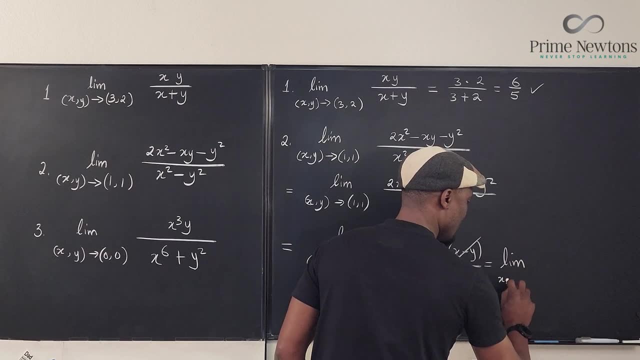 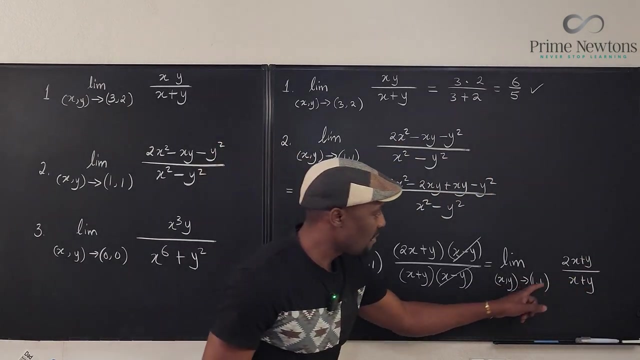 the toughest part of this is just factoring, which is an algebra skill. okay, so if we take this out, we take this out, what we have left is going to be the limit as the point x- y approaches. one one of this is what is left: 2x plus y, divided by x plus y. well, we can easily plug in our one for x. 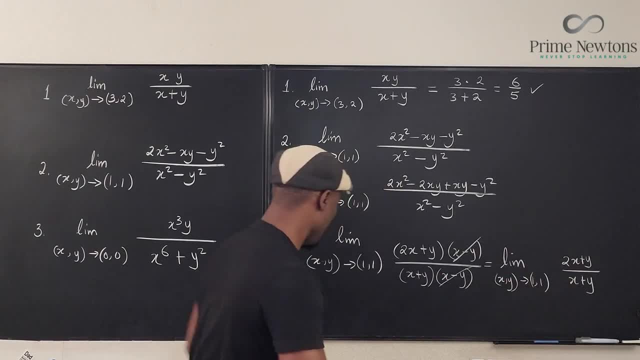 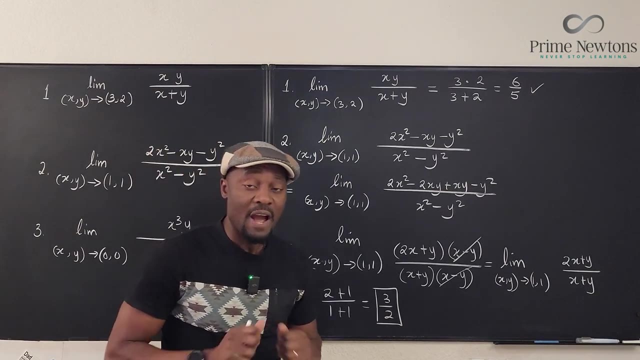 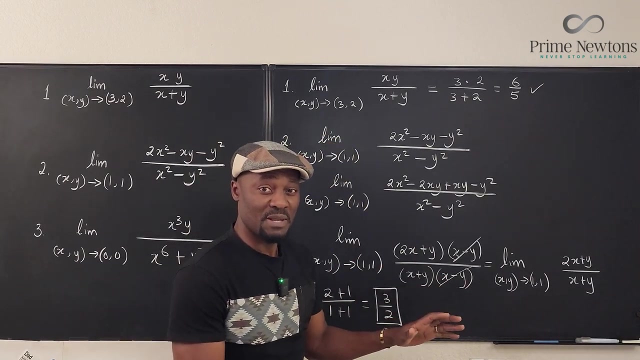 one for y, we're going to end up with two. so this is equal to two plus one over one plus one, which is 3 over 2.. So the limit of this is 3 halves. Okay, now there are other strategies you can use to compute your limit, but if it is obviously algebraic manipulation, just do it. 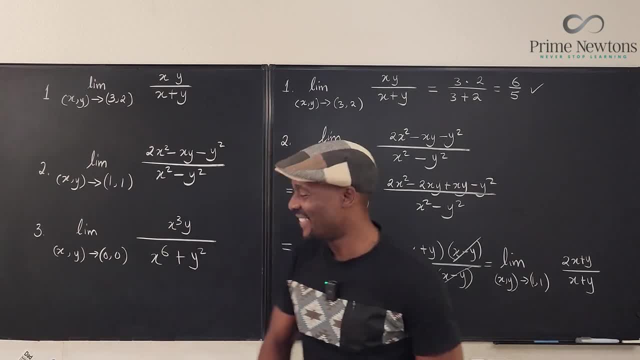 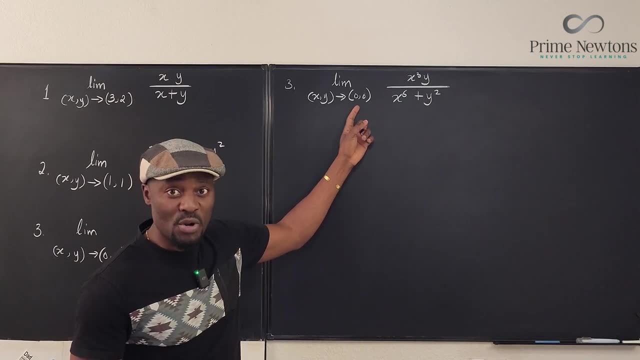 It is usually easier, or maybe sometimes tougher. Okay, let's go to the third one. This one is a little tricky because the finite point we have is the point 0, 0. And if we plug in 0 for each of x. 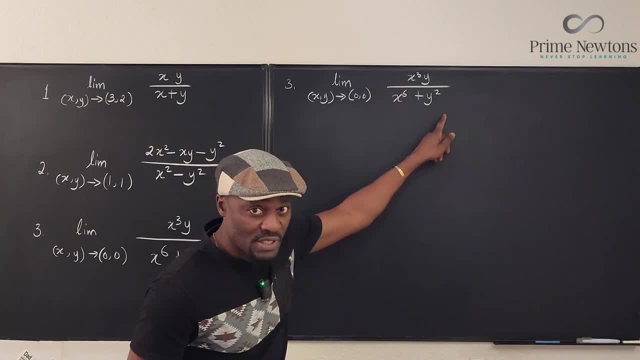 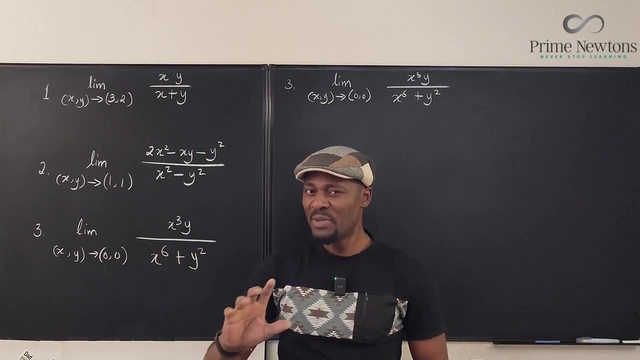 and y, you're going to end up with 0 over 0.. Now, that's a similar situation to what we had here initially. So, remember, the next thing you're supposed to do is to say: I need to factor the top. 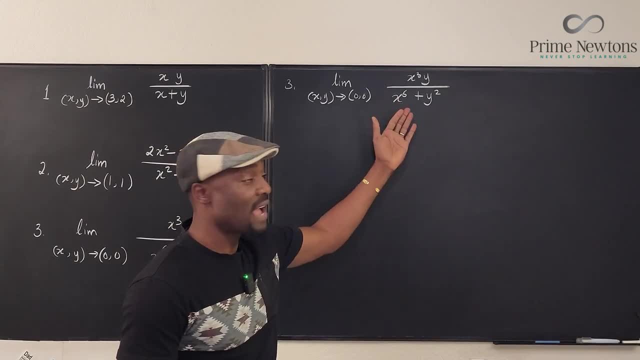 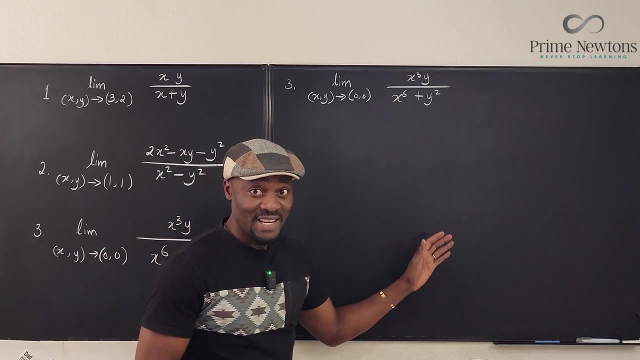 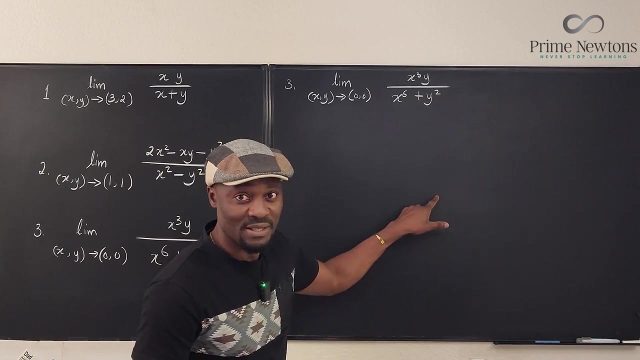 and the bottom. Unfortunately, there's nothing you can factor here, But this is actually a very nice one because it is plain and simple. What I mean by that is, on a plane, you have many different directions you can approach a point, So you can tell yourself instead of me. 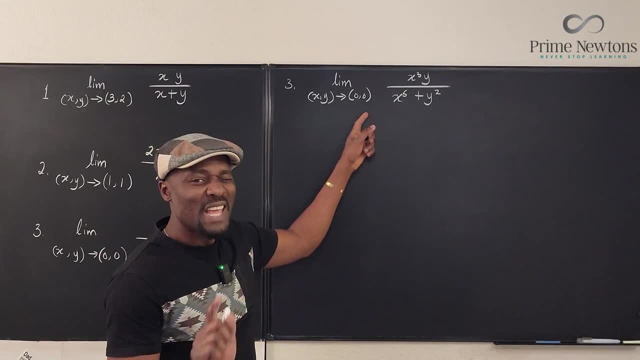 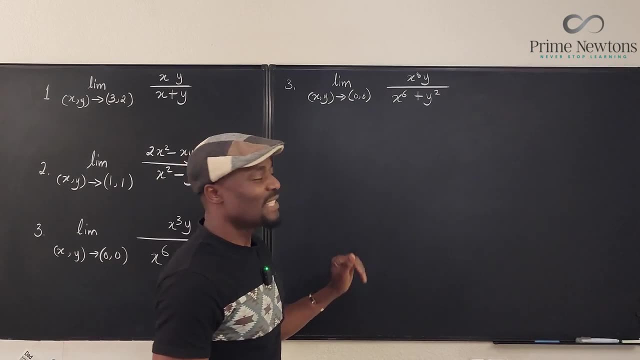 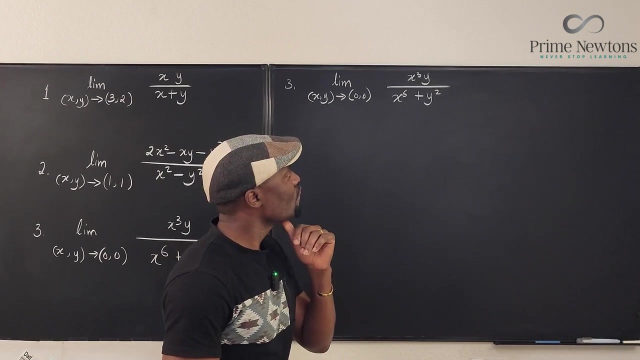 just getting stuck with 0, 0,. what if I tell myself I'm going to approach this point through a function that gets rid of either of the two variables? And how do you do that? You just have to do a substitution and say: what if I say: let y be equal to x, cubed. 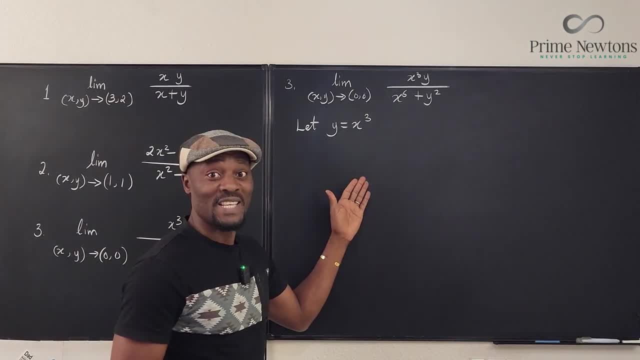 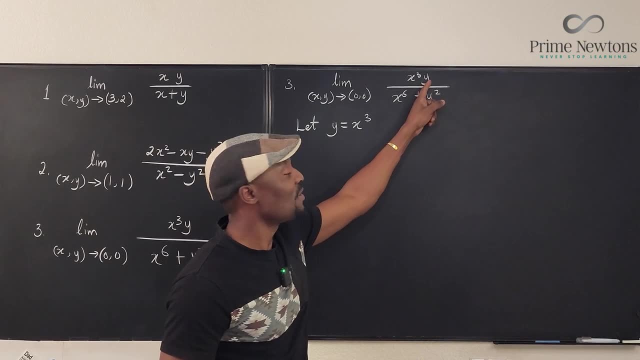 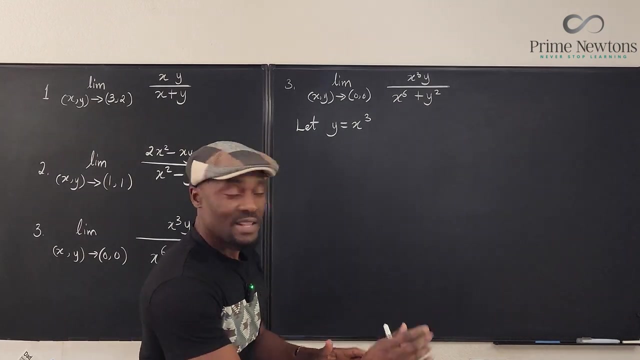 You see, this makes life a lot easier, because if y is equal to x cubed, you see, that's what is standing next to it. So instead of you writing y, you just replace y with x cubed. And instead of writing y here, you replace it with x cubed, Because it's a plane. this is a function that. 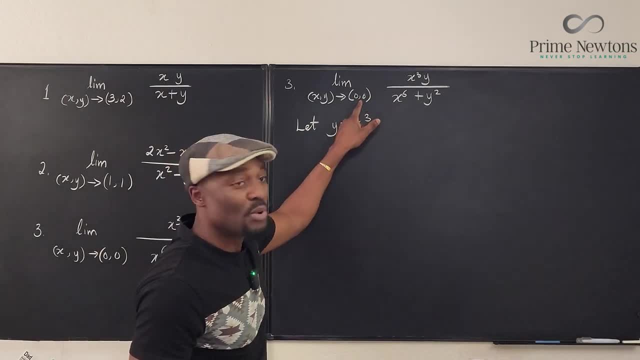 will go through the point 0, 0.. How do you know it's going to go through the point 0, 0?? Well, when x is 0, y is 0. So you know that function is a valid function. 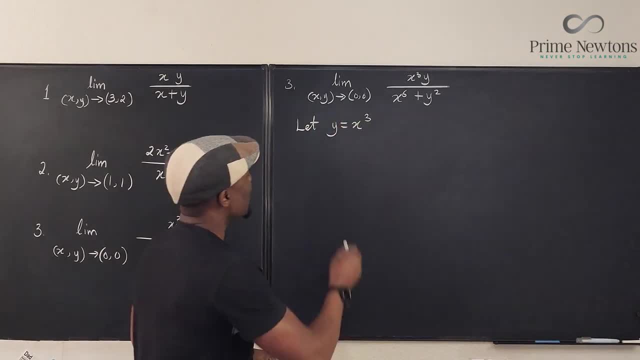 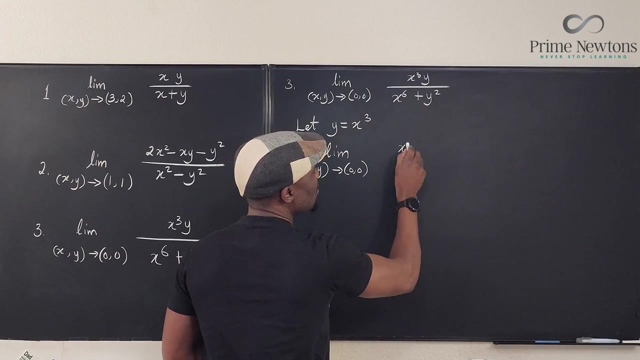 So, if you use it here, what do you end up getting? You're going to get the limit as the point x, y approaches, 0, 0.. This is now going to end up becoming, instead of you writing y, you're going to end up with x cubed times x cubed, which is going to be x to the 6th. 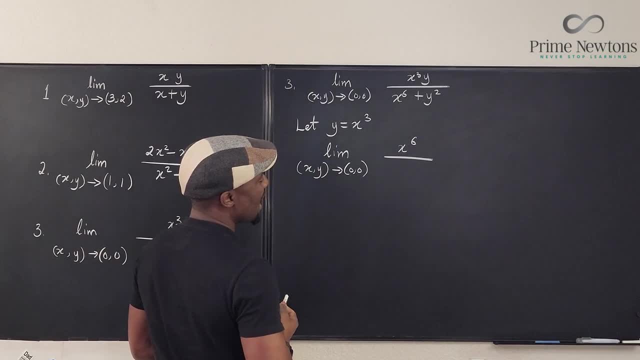 And on the bottom, what are you going to have? You're going to end up with: um wait, let's write this first, because that's not correct. And then this is: x to the 6th plus y squared will become the limit. 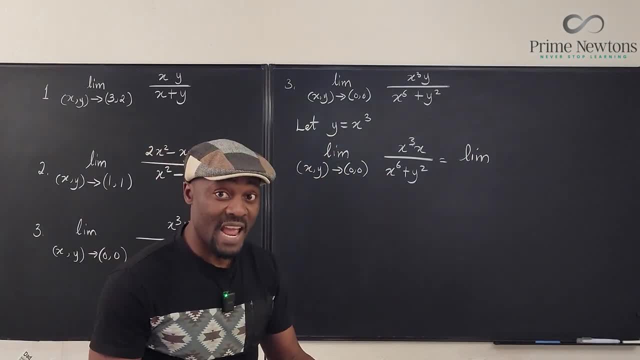 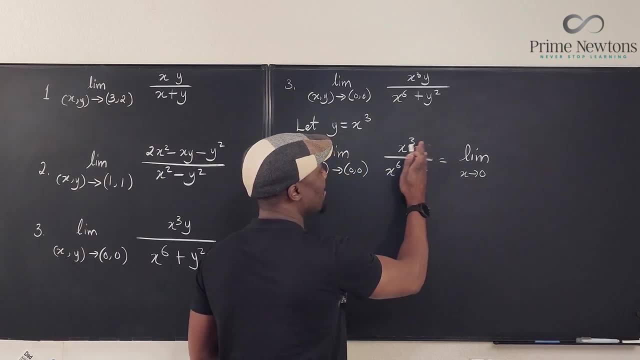 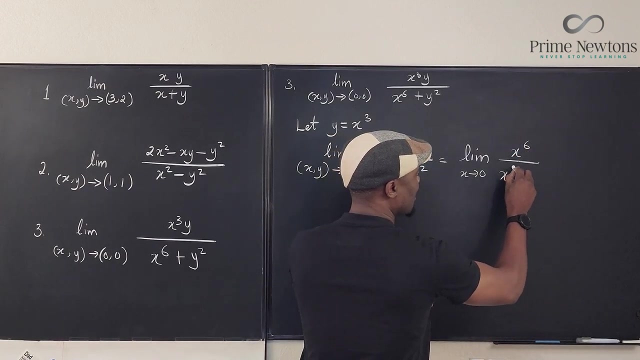 Because now the new function you're going to have will only contain x, So you just have to say the limit as x approaches 0. And then you're going to have: oh, this is y, come on. So you're going to have x to the 6th over. this is going to be x to the 6th plus, this is going to be x cubed. 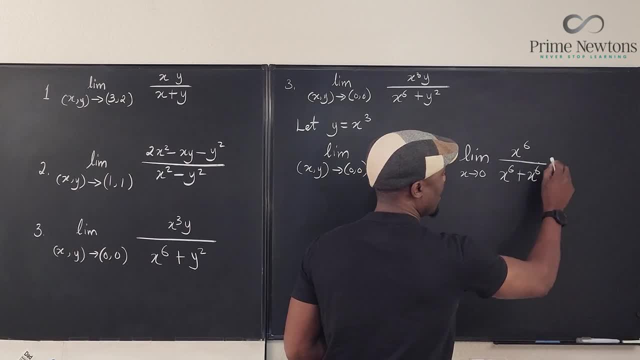 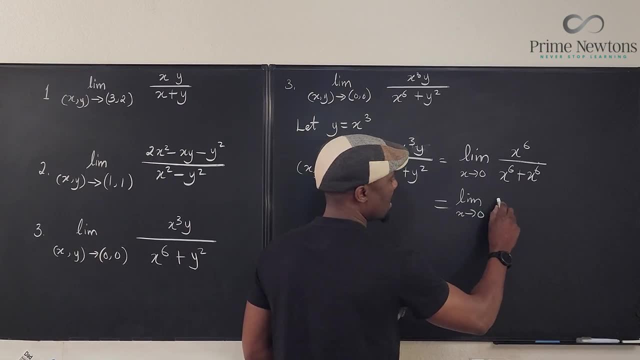 squared, which is x to the 6th also. Huh, And this is going to work out to be the limit as x approaches 0.. And this is going to be x to the 6th over 2x to the 6th, which is going to be the limit, as x goes to 0, of 1 over 2,. 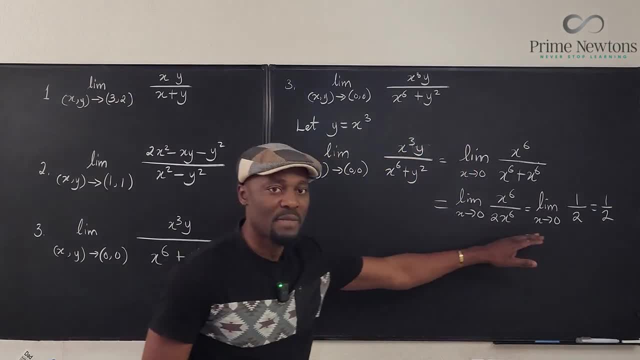 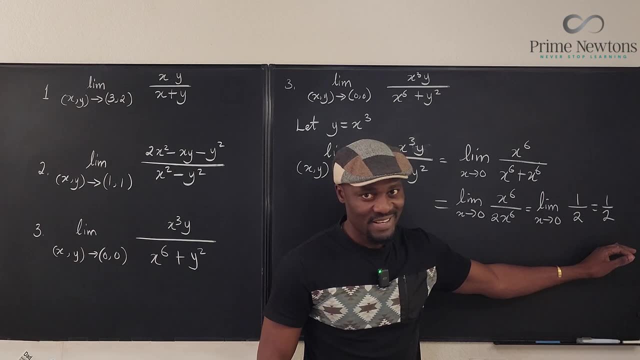 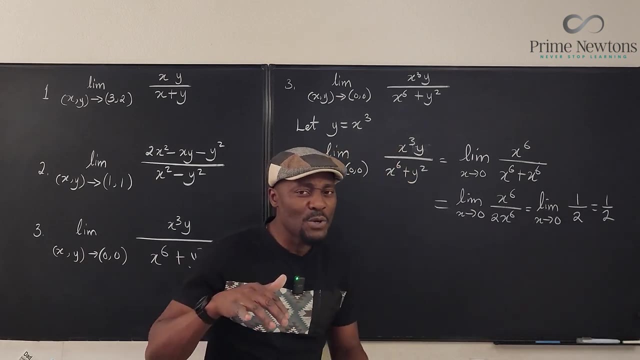 which is 1 half. So you get 1 half. if you do this strategy, Does that mean this is the limit? No, That's the problem with multivariable functions. You don't know whether this is the limit because remember how we used to do: the limit from the left has to be equal to the limit from the 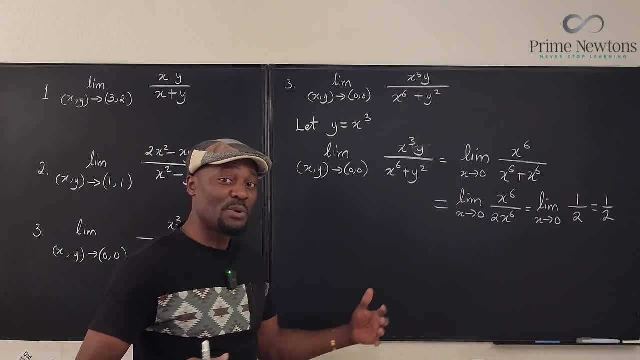 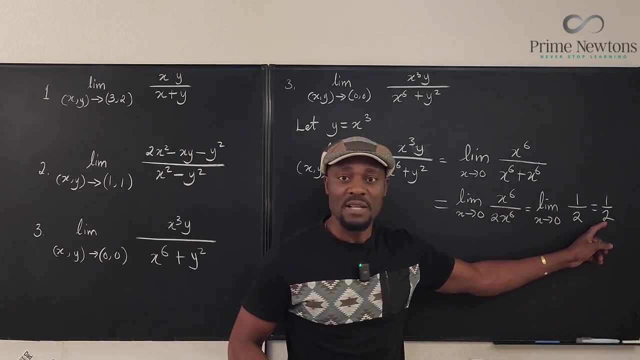 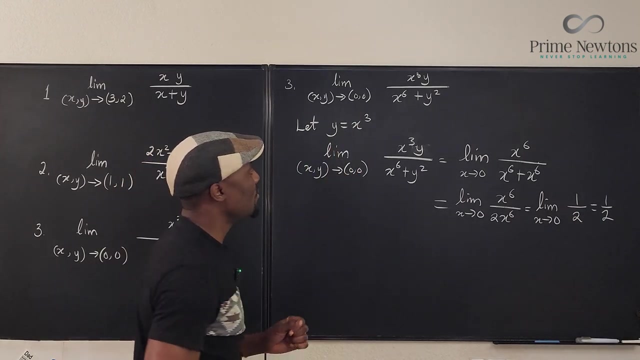 right. So the same thing. you have to pick multiple directions and make sure that all the directions you will ever pick will always give you the same answer. So let's try to find another direction. We just did let y be equal to x, cubed. 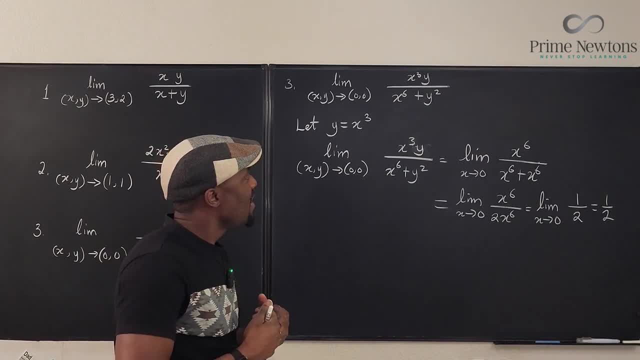 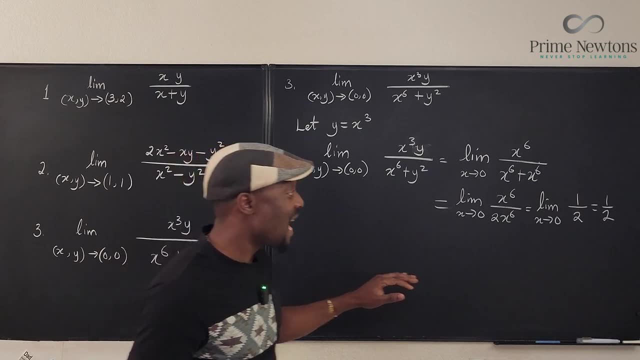 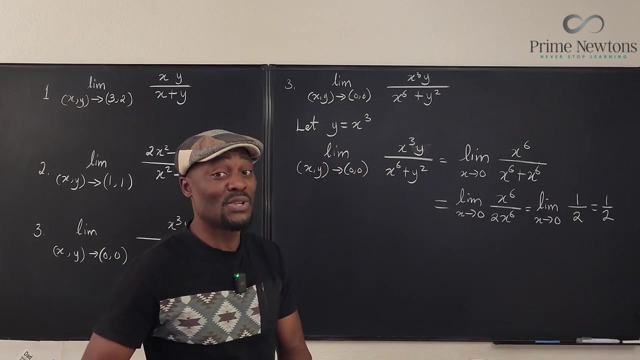 We can do something else. What if we say let x be equal to y? That's another direction. So if we now find another direction and the answers are not the same, then definitely the limit does not exist. If the answer is the same, we may have to try a third one, just to confirm. 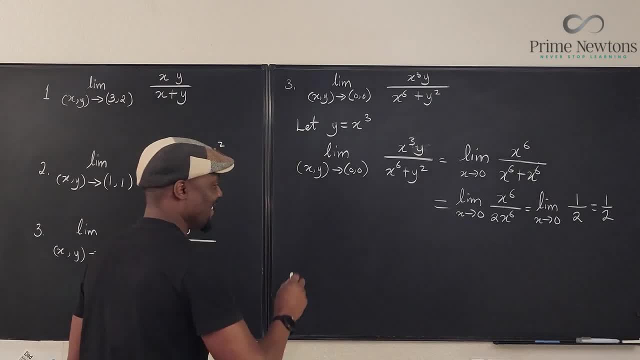 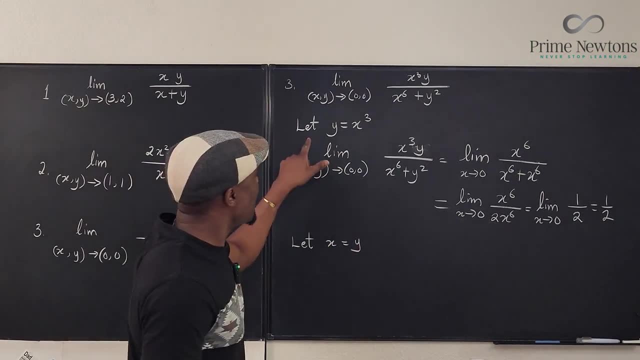 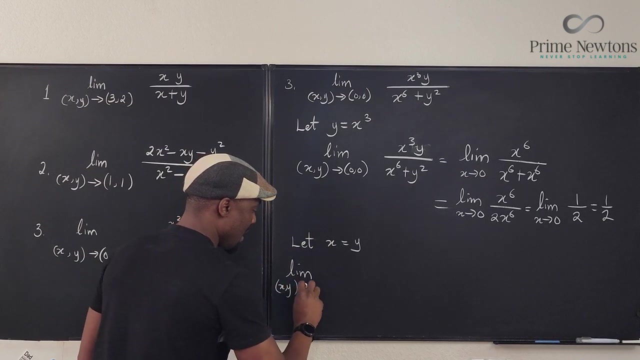 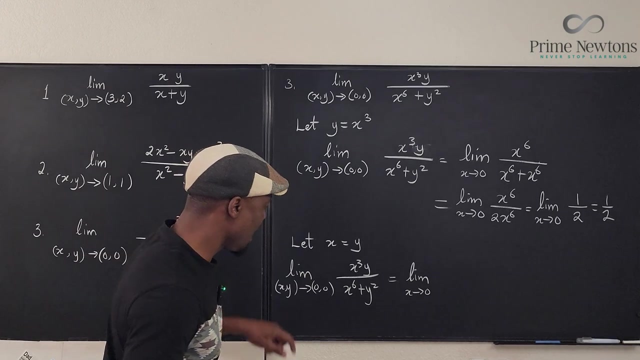 Okay, maybe not the best method. Okay, so let x be equal to y. So if x equals y, the limit can become: you have the limit as xy approaches 0, 0 of what we have. x cubed y over x to the sixth plus y squared will become the limit as x goes to 0.. If x is equal to y,